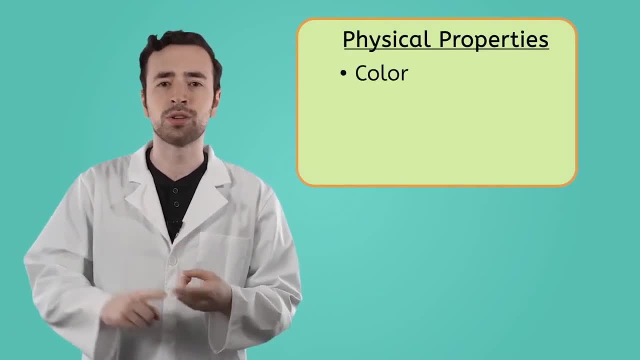 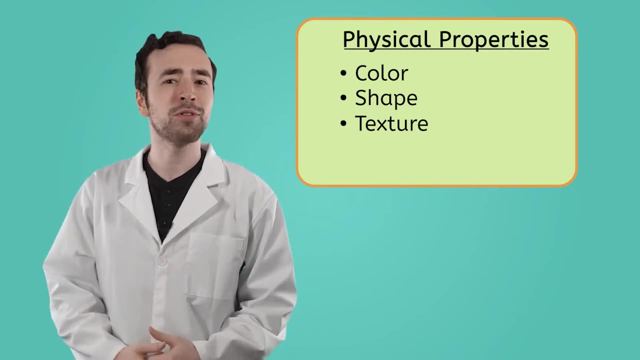 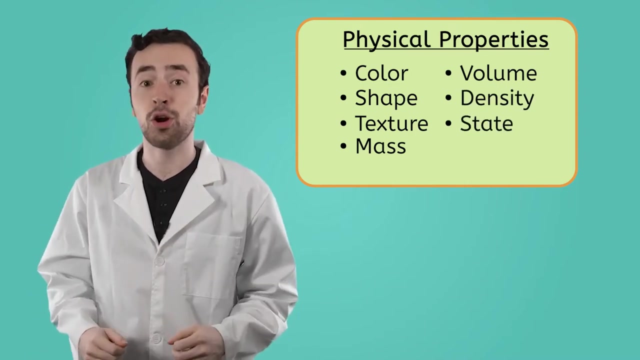 the physical properties we've talked about so far are things like color, shape, texture, But did you know that a lot of the things we've learned about in this unit are also physical properties? Yep, mass volume, density and state of matter are all physical properties as well. They can all be. 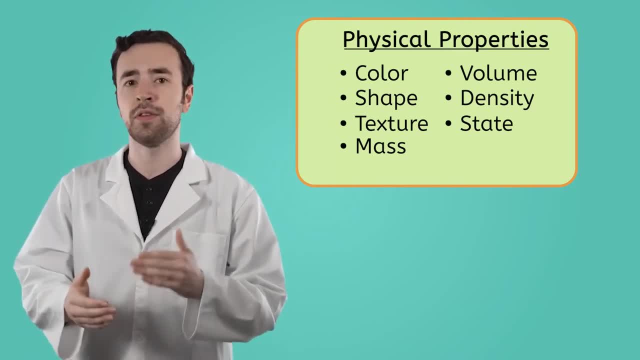 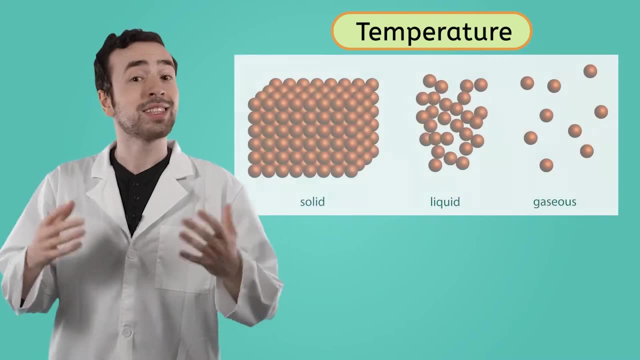 observed without changing the identity of the matter. So I can observe this. chair, see that it's of the matter. Another physical property of matter is the temperature at which it changes. states, State changes are a physical property because they don't change the identity of the. 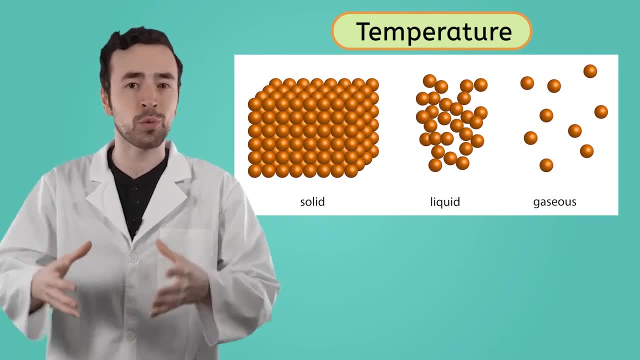 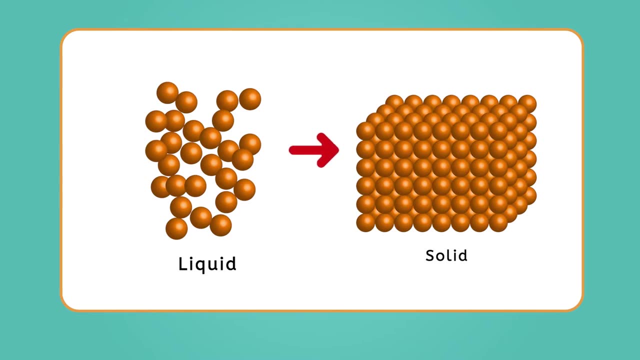 matter. It's still the same matter. its atoms are just rearranged in a different way. The temperature at which matter changes from a liquid to a solid is called its freezing point, And the temperature at which it changes from a solid to a liquid. 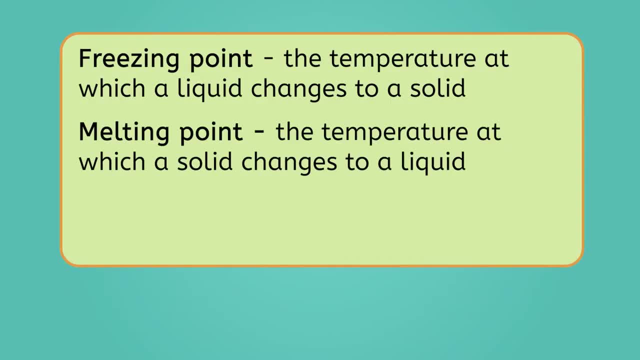 is called its melting point. The freezing point and melting point, of course, are the same temperature. After all, it's the exact temperature at which that specific piece of matter would change. state For water that temperature is 32 degrees Fahrenheit or zero degrees Celsius. 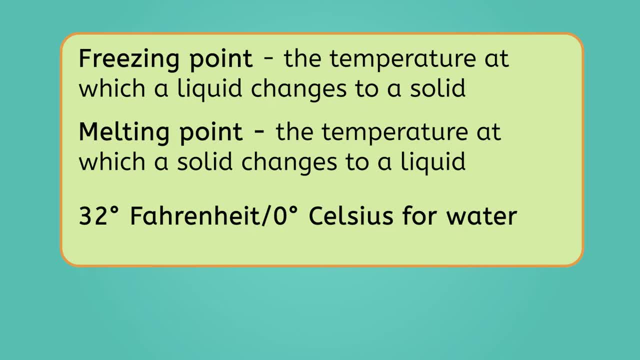 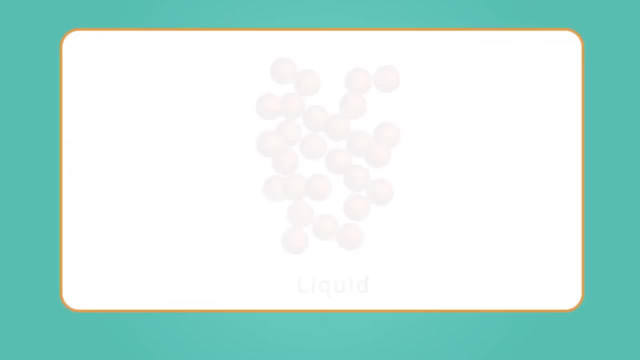 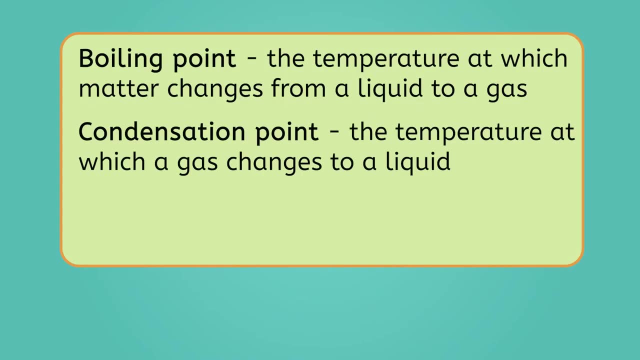 Anything below that temperature and water will freeze. Anything above that temperature and water, or really ice, will melt. The temperature at which matter changes from a liquid to a gas or a gas to a liquid is called its boiling or condensation point, That's. 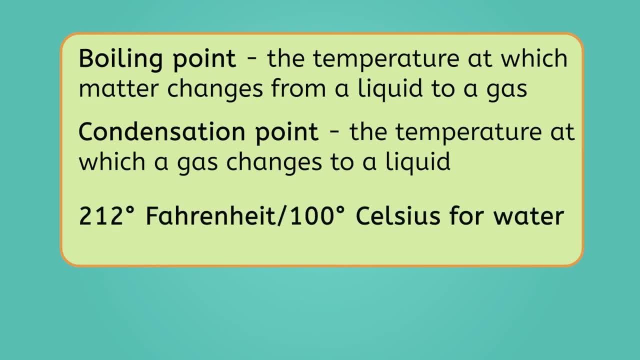 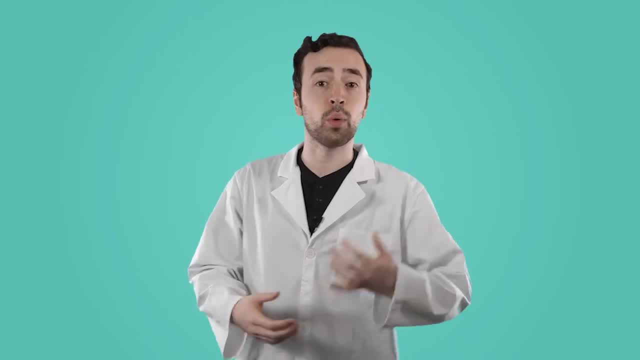 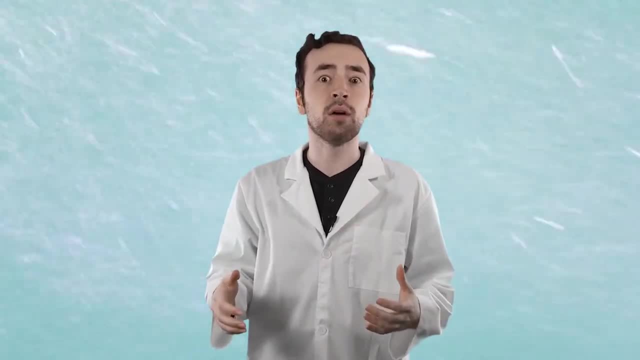 212 degrees Fahrenheit or 100 degrees Celsius for water. Different kinds of matter will have different melting and boiling points. For example, the oxygen gas that's in our atmosphere won't condense into a liquid unless it's really cold like almost. negative 300 degrees Fahrenheit. In case you're worried, the lowest temperature ever recorded outside on Earth was only negative 128 degrees Fahrenheit, So the oxygen gas around here will always be probably a gas. Phew, I gotta pay attention to when the materials I'm using for my rocket freeze or boil. 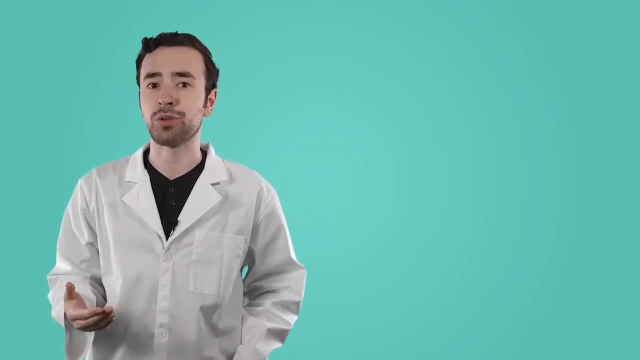 Another property of matter that I should pay attention to is something called solubility. the ability for matter to dissolve, COLLAPSE, converse, natural, immediately omits CONTROL MECHALOGY RESOL하는 on the source. s tenemos que el material no tiene dignidad de place en suистişi트를. 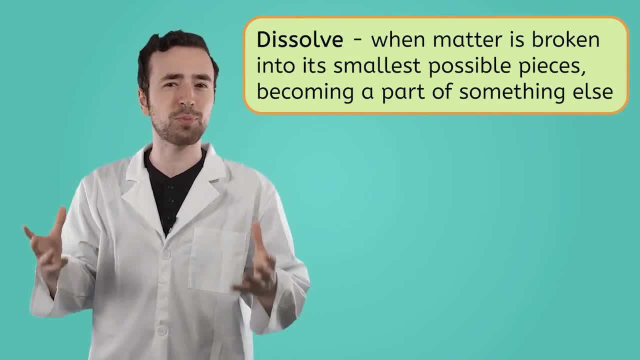 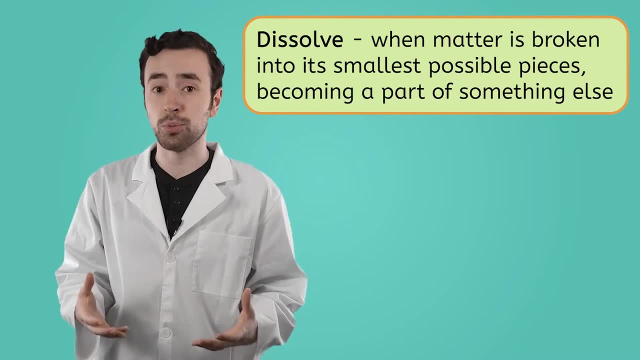 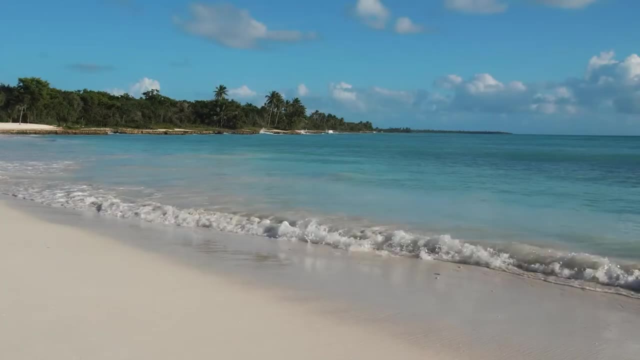 Matter dissolves. it breaks down into the smallest pieces of itself and becomes part of something else. For instance, some matter is soluble in water, meaning it will dissolve in it, and some matter isn't. For example, think of the last time you went to the beach. 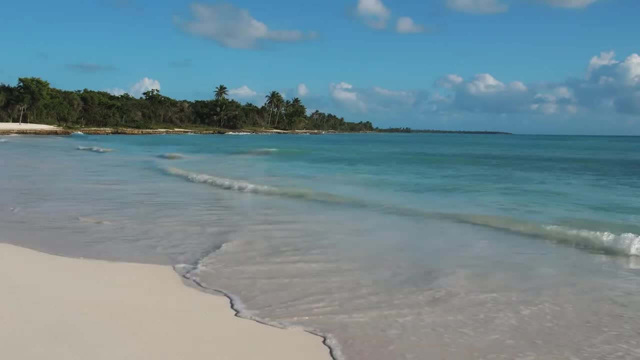 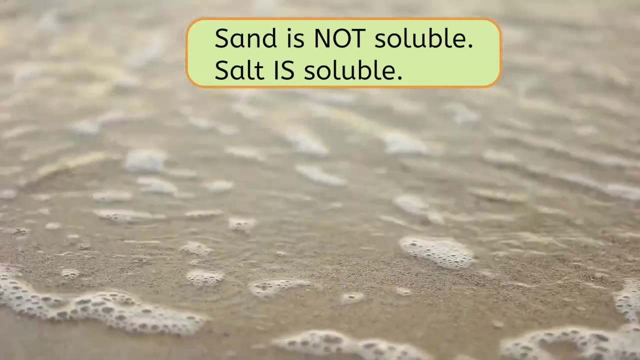 I bet you got sand everywhere. That's because sand is not soluble in water. It doesn't dissolve. Salt, on the other hand, is soluble. The salt in the ocean is dissolved, so you can't see it and it's spread throughout. 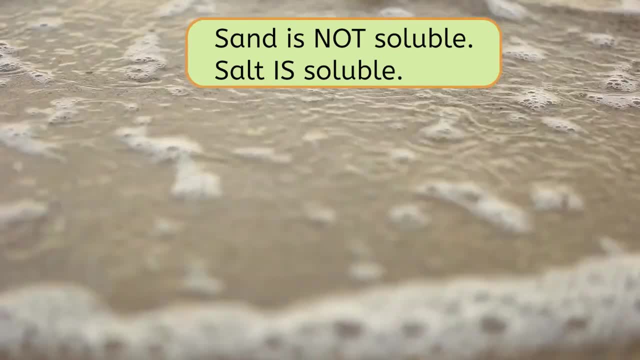 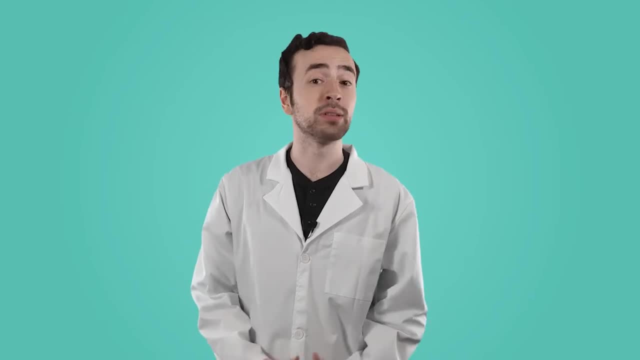 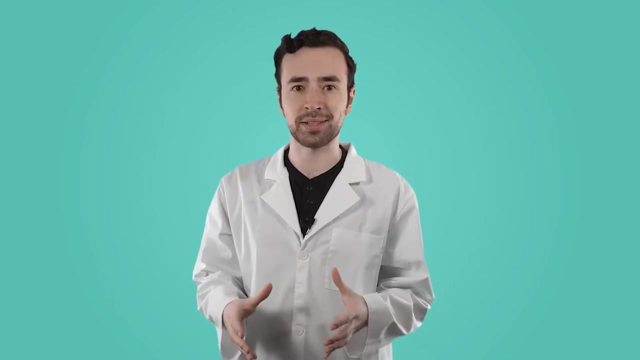 the water. It doesn't settle on the seafloor like the sand does. I'll definitely keep solubility in mind when I'm building my rocket, But a physical property that's probably even more important than that has to do with magnetism. 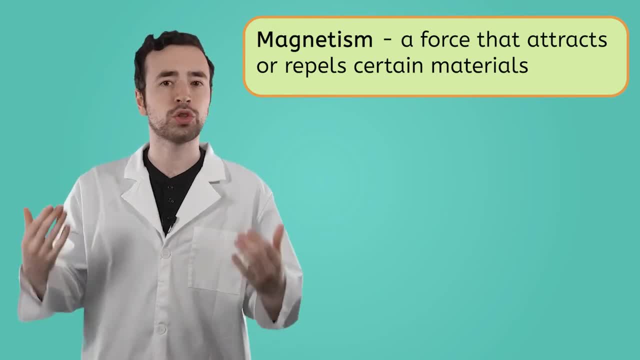 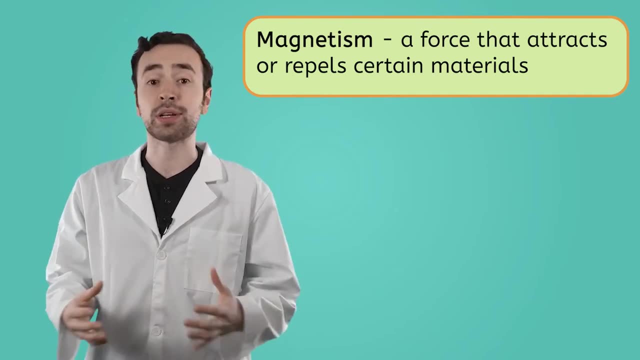 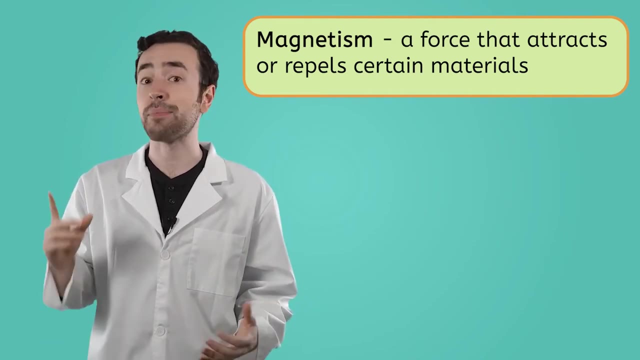 Magnetism is a force that attracts or releases. It repels certain materials. Whether or not an object is magnetic is a physical property. For example, iron, nickel, cobalt and steel are all magnetic metals, meaning that magnets will attract them. 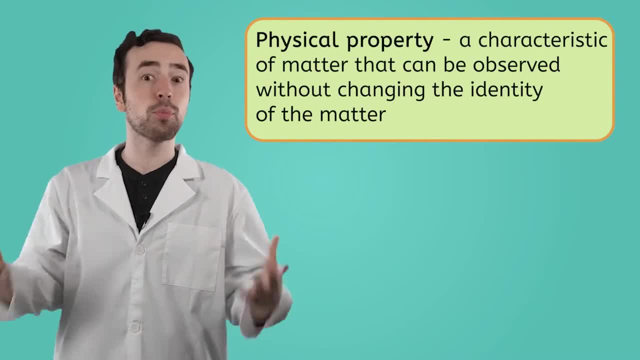 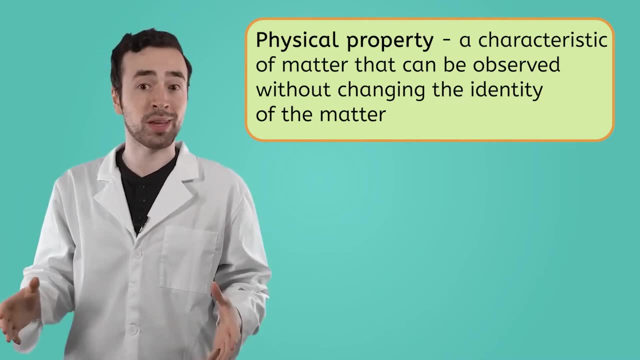 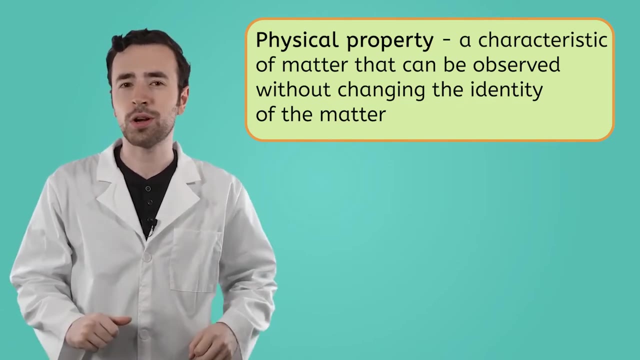 So the physical properties of matter are all the properties that we can observe without changing what the identity of the matter is. Trust me, There are tons more physical properties that we just haven't talked about, But what happens when the matter we're observing does change? 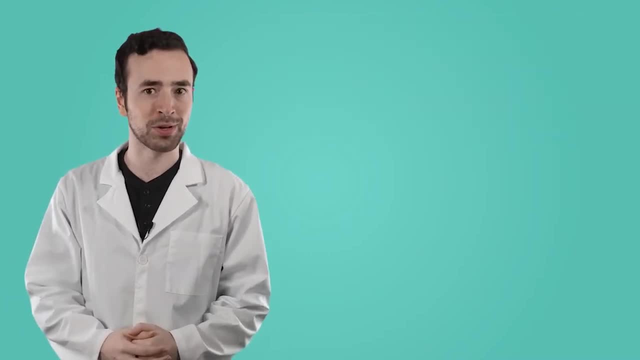 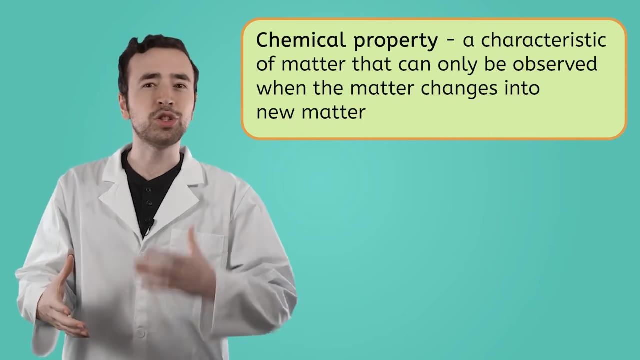 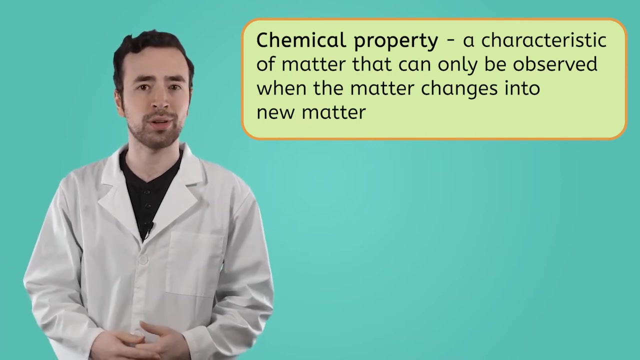 Well then, we've got some chemical properties to observe. A chemical property is a characteristic that we can only observe when the matter changes into a new kind of matter. One of the ways that matter can change is through a chemical reaction: Reactivity. 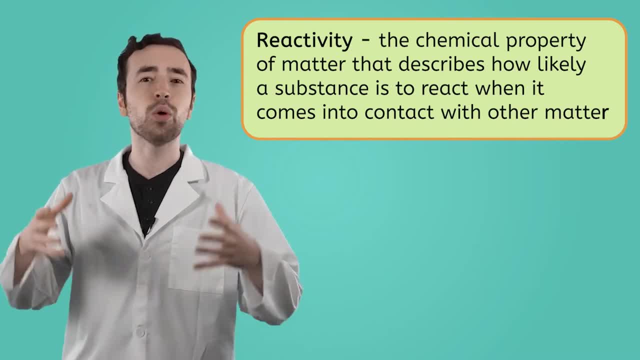 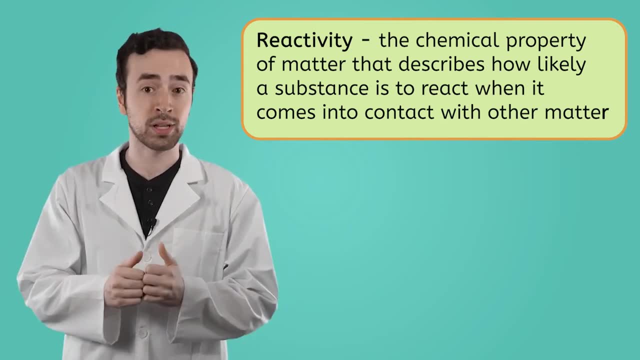 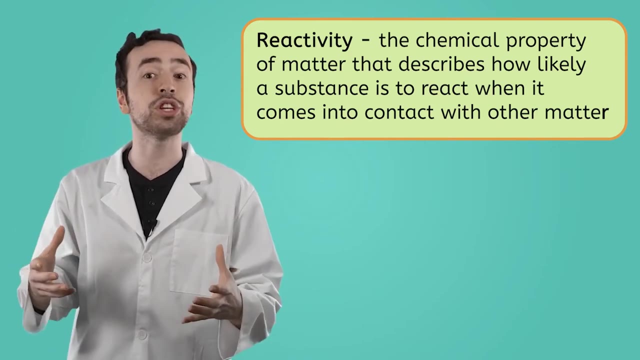 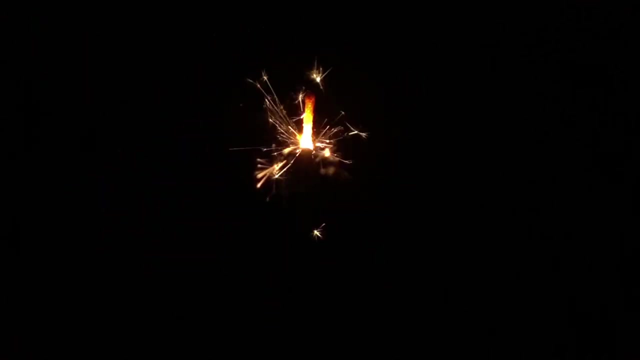 Reactivity, A chemical property of matter that describes how likely it is for a substance to react when it comes into contact with another substance. When matter reacts, it changes into a new kind of matter and energy is released. For instance, the metals on the end of a sparkler are highly reactive.